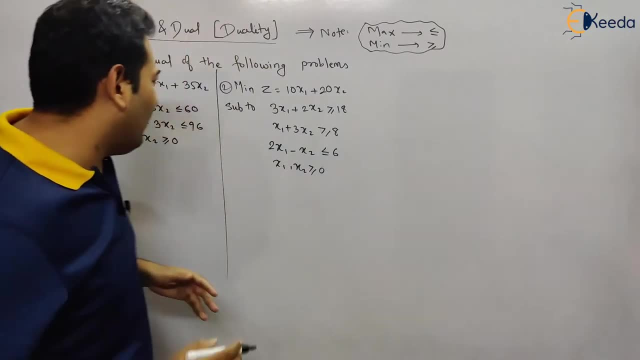 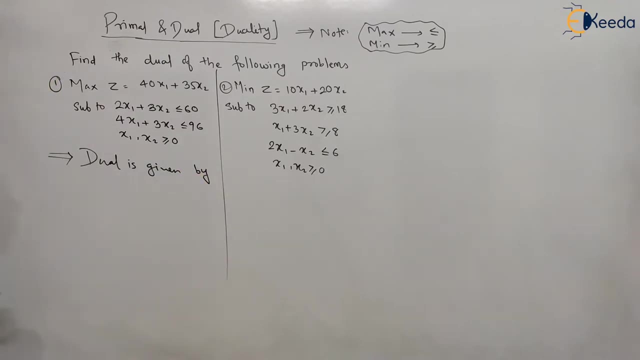 primal is in the correct form. Now we can form its dual. Dual is given by. So see the way I am writing down the dual. Maximize, its dual will become minimized. If it is minimized, its dual will become maximized. W is: 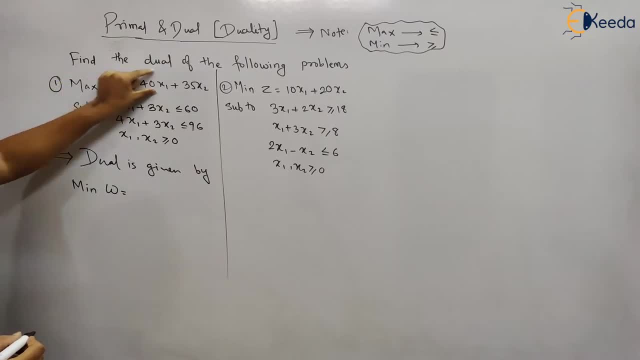 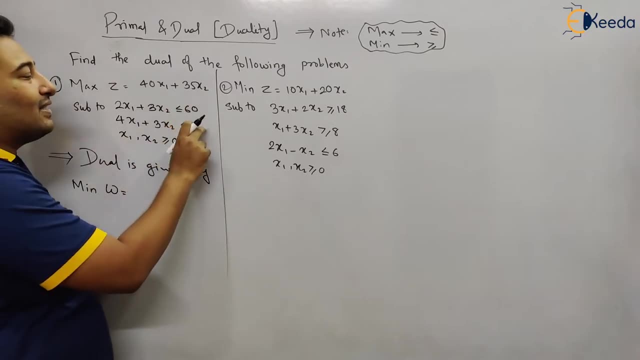 equal to the objective function. See, this is called objective function and these are your constraints. Objective function will be formed based on the right hand side of the constraint. See, you need to remember the steps. Objective function will be formed on the basis of the right hand side of the constraint. So there are two. 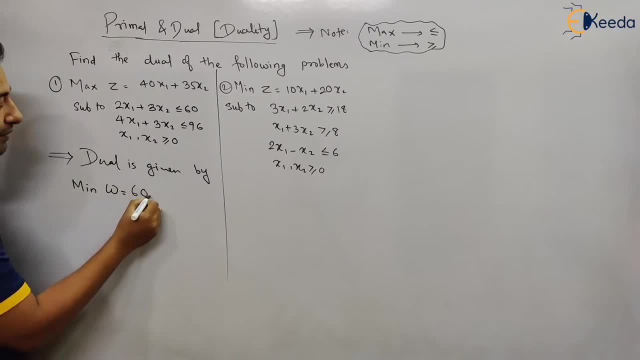 constraints, And here we have 60 and 96. Therefore, it will be 60y1 plus 96y2.. 60y1, 96y2.. Subject to See the way I am writing the constraints, They will be formed based on the. 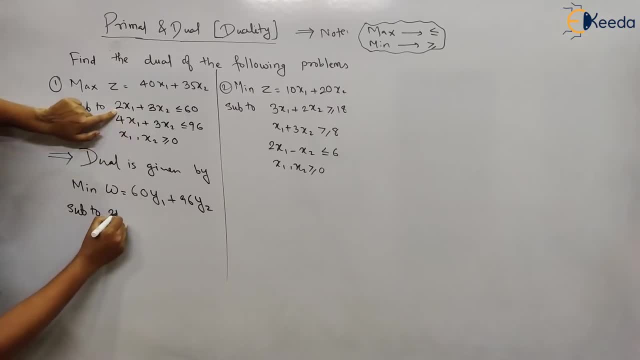 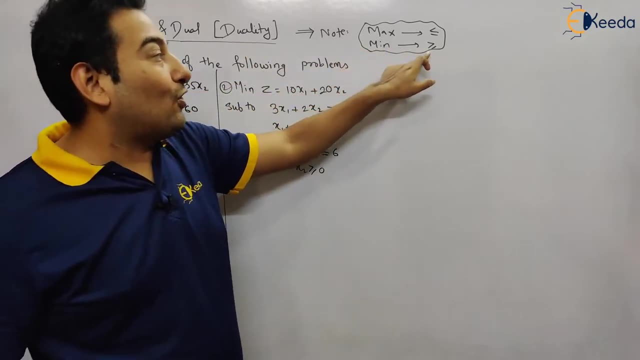 coefficient of x1.. See, here we have 2.. So that is 2y1.. Here we have 4.. So that is 4y2.. And since it is minimized for minimize, all the constraints should be greater than equal to, So that is greater. 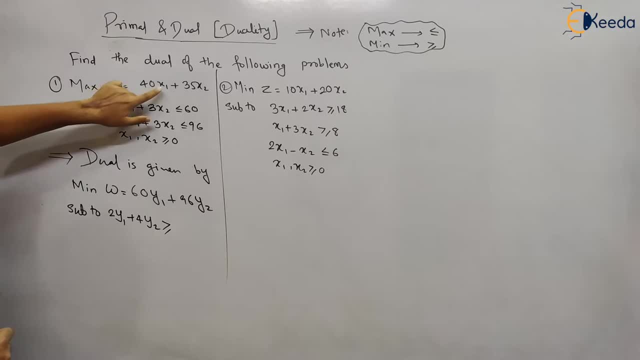 than equal to 2y1,. 4y2 greater than equal to In objective function. with x1, we have 40.. So that is 40.. Next, the second constraint will be the coefficient of x2.. So that is 3y1.. 3y2 greater than equal to. With x2, we have. 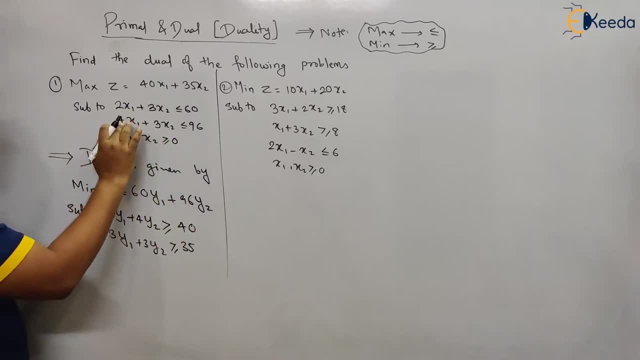 35.. So that's it. There are only two constraints, Two coefficients of two variables: x1 and x2.. So we got two constraints And finally y1, y2 greater than equal to 0.. This is by default. 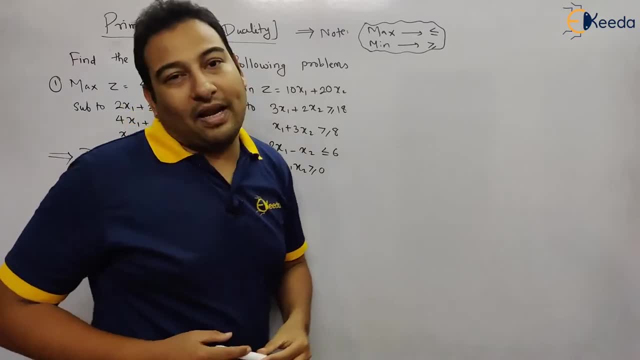 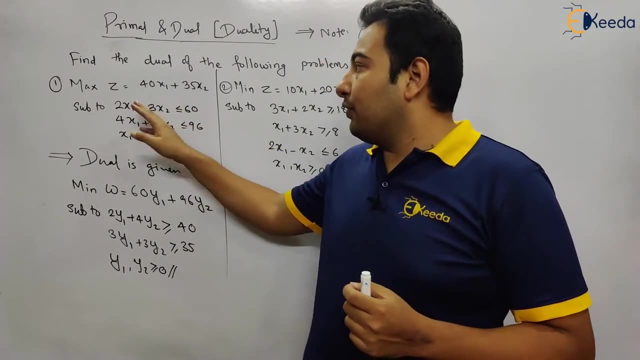 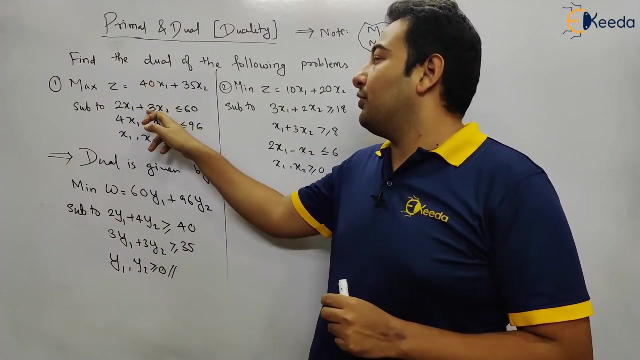 So this is the primal dual of the above primal. Is this clear? So it's very clear from this how to write the dual For objective function, whatever will be the RHS of the constraint that we're going to consider, And for writing down the constraint, we're going to consider these coefficients. 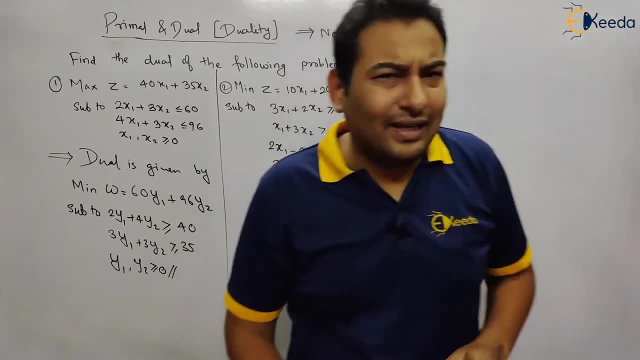 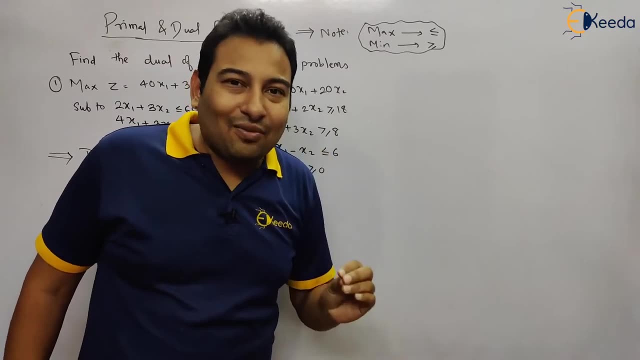 Let us discuss the next example, problem number two, and it will be very clear. So let us discuss problem number two. This is your primal. Whatever problem is given, these are primals. So let us check whether the primal is in the correct form or not, And what is. 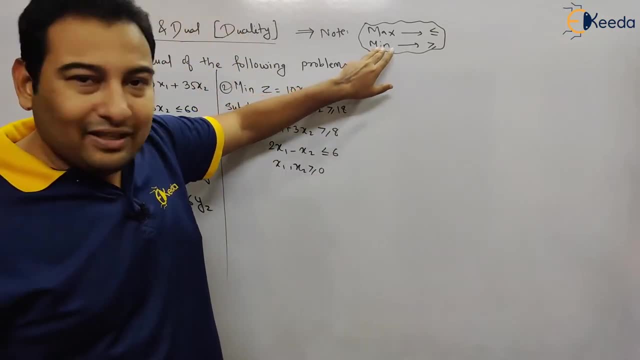 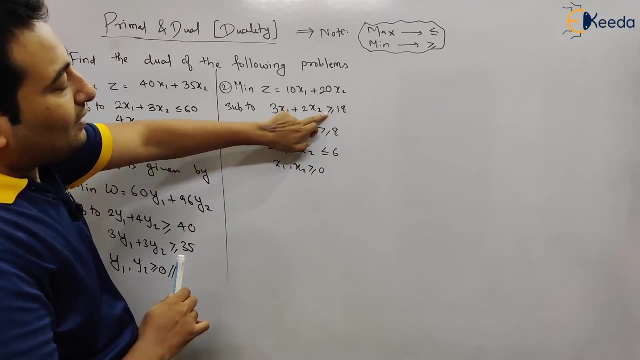 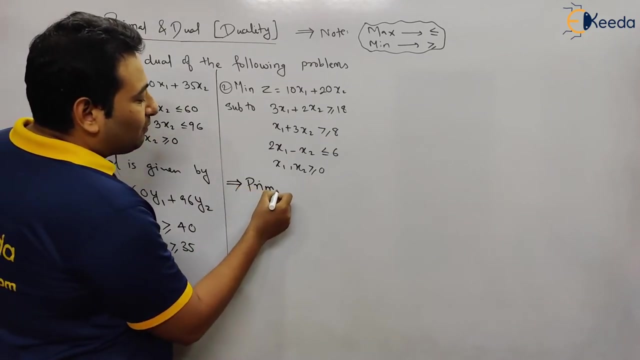 the condition for primal to be correct. If it is minimized, all the constraints should be greater than equal to. So let us check: here The problem is minimized And these two constraints are greater than equal to, but here it is less than equal to. Therefore, first of all, you need to change this. 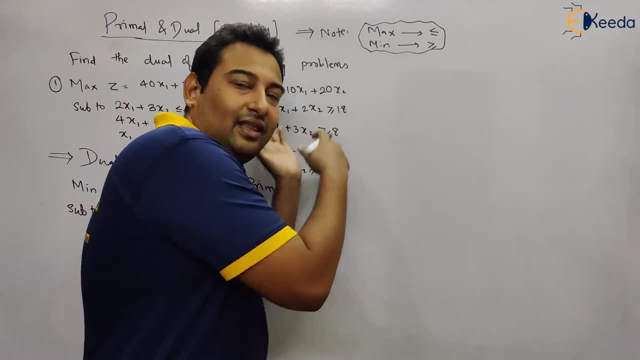 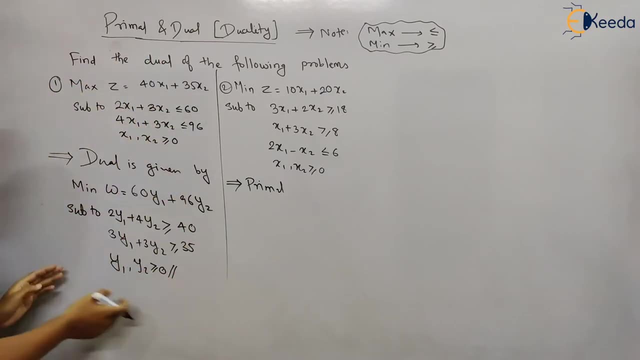 primal. First of all, your primal should be ready. Once your primal is ready, then you can convert it into dual. Here the problem was already. Primal was already correct. Therefore we directly found out it's dual, So primal is. 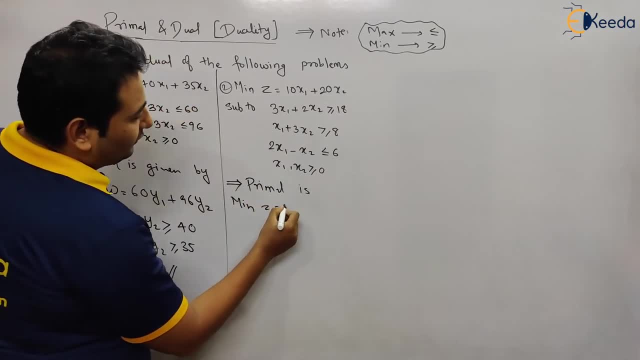 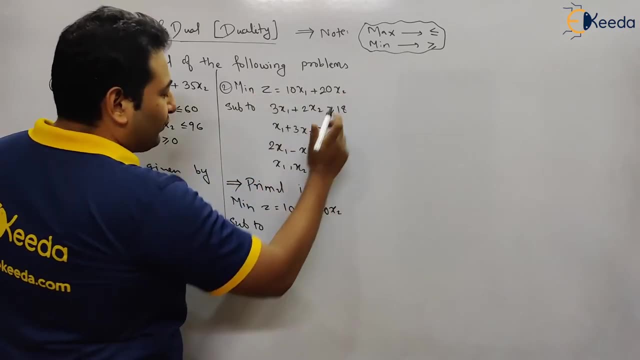 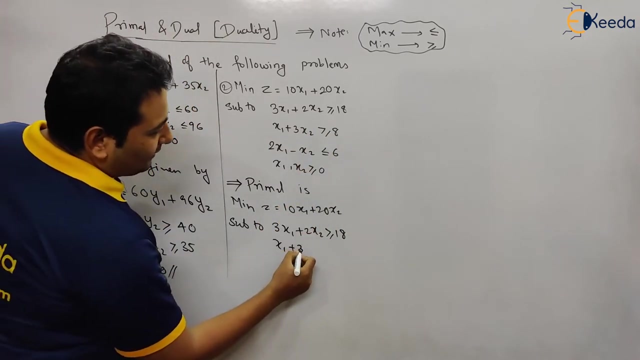 minimized. Z is equal to 10x1, 20x2,. subject to The first constraint is perfect, So no need to touch it. Keep it as it is. Second constraint: also keep it as it is The third constraint. there is a problem. Since it is minimized, all the constraints should be. 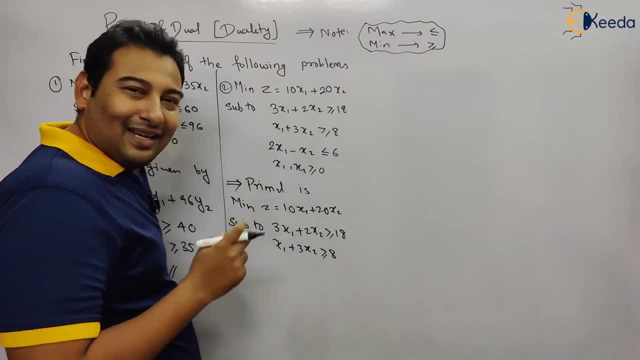 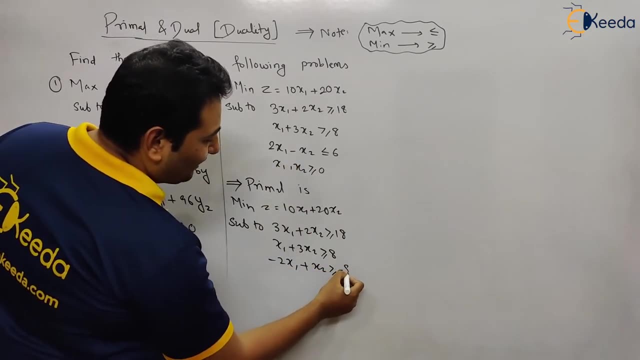 greater than equal to. Therefore you need to minimize it. So let us check here. So we multiply the third constraint with the minus sign and convert it into greater than equal to. So minus 2x1 plus x2 greater than equal to minus 6.. And finally, x1, x2 greater than equal to 0.. 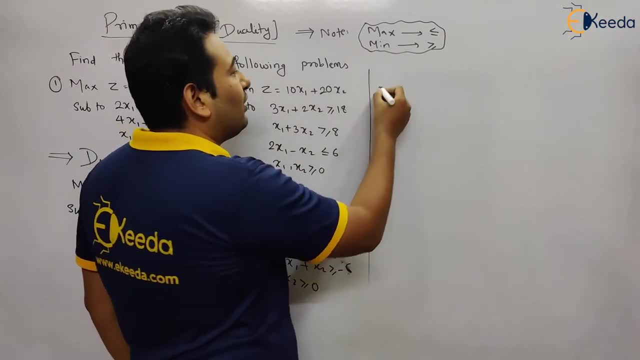 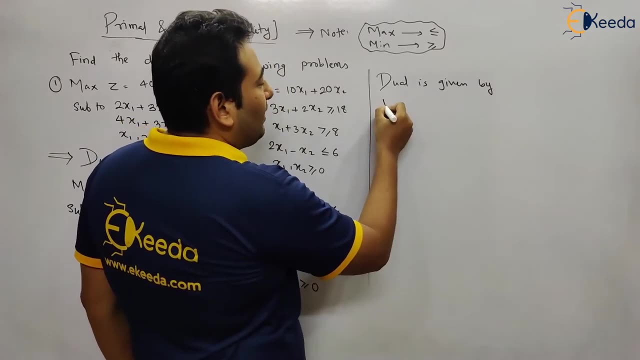 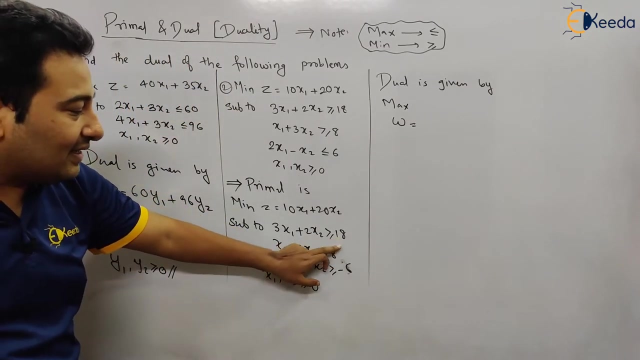 Now your primal is ready, which can be converted into dual. So dual is given by minimized is dual will be maximized. W is equal to See here. Check the right hand side of the constraint. So here it is 18, 8 and minus 6.. 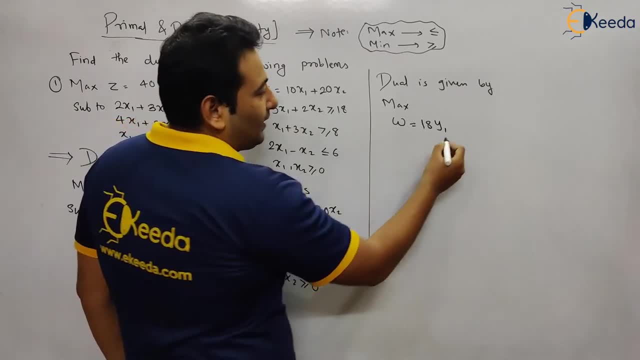 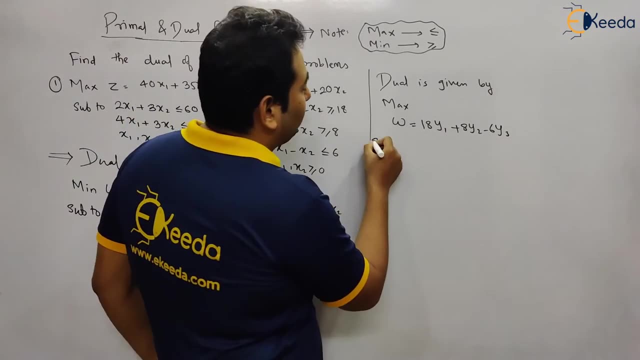 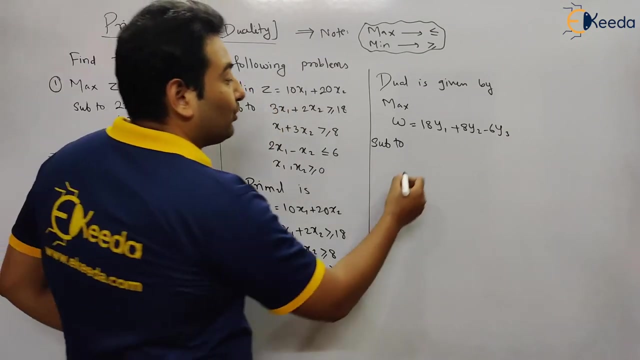 So 18y1 plus 8y2 minus 6y3.. 18, 8 and minus 6, subject to With x1, we have 3.. Here we have 1.. Here we have minus 2.. So that is 3y1.. Then we have 1.. So that. 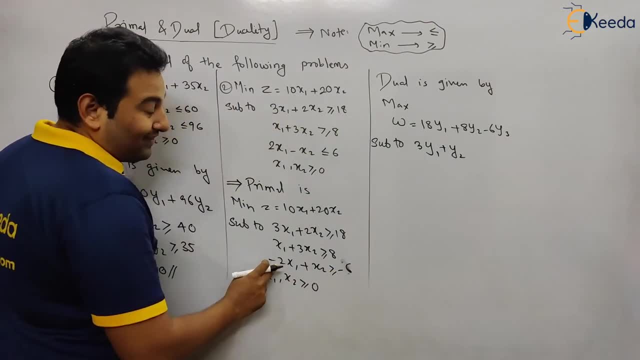 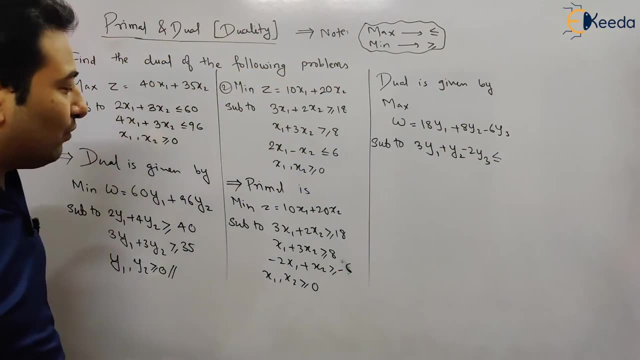 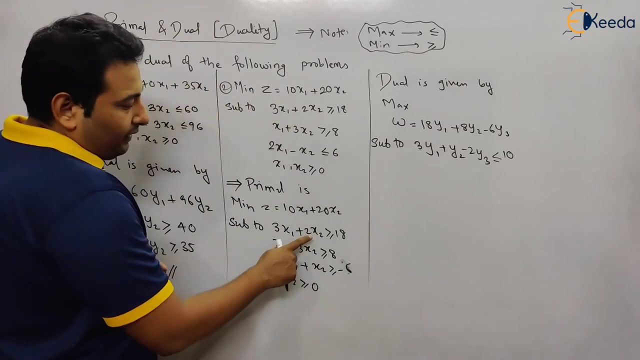 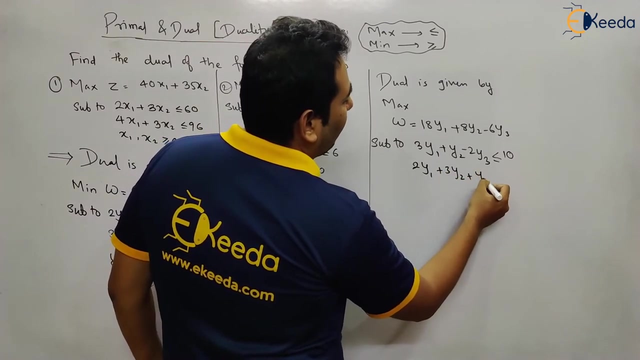 is y2.. These are the coefficient of the first constraint, That is minus 2y3. And since it is maximized, it will be converted into less than equal to less than equal to 10.. Next, with x2, we have 2, 3 and 1.. So 2, 3 and 1, less than equal to, With x2 in the objective.